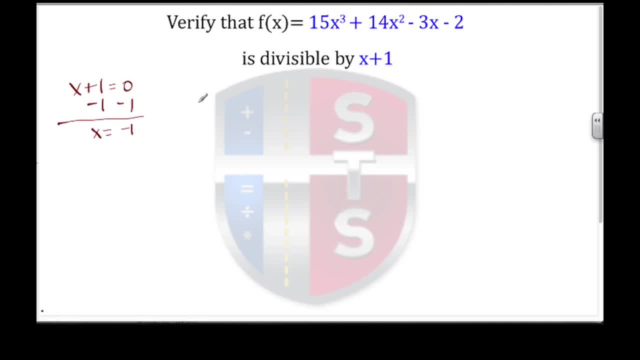 End up subtracting 1 from both sides and figuring out that x, in this case, would be a negative 1.. So that there is our divisor. Then we continue by taking the coefficients of each one of the terms in our function f of x. 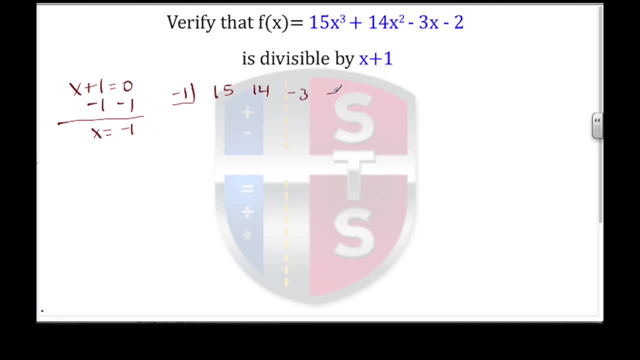 So 15, 14, negative 3, negative 2.. And we begin by bringing down this first coefficient of 15.. So negative 1 times 15 would give me a negative 15.. 14 minus 15 would give me a negative 1.. 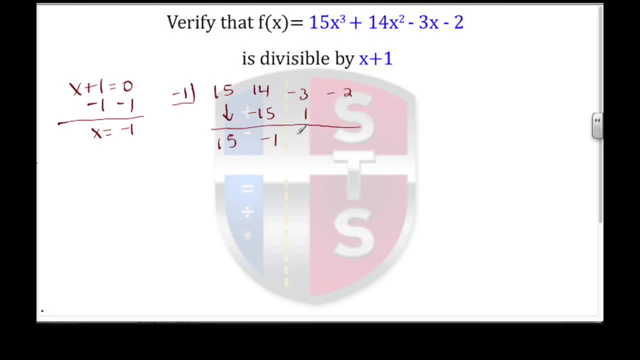 Negative 1 times negative 1 would give me a positive 1.. Negative 3 plus 1 would give me a negative 2.. And then negative 1 times negative 2 would give me a positive 2.. So here we see, we have a remainder of 0, which does show us that x plus 1 is indeed a factor. 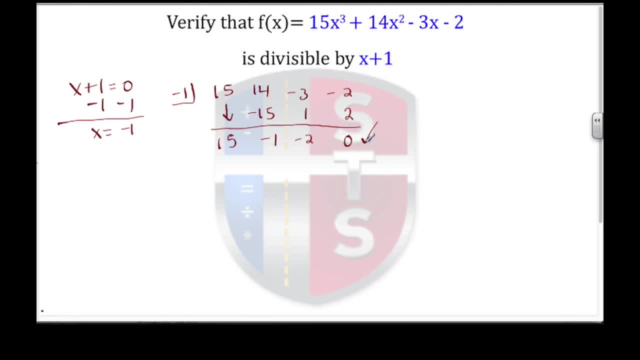 Or another way, stated can be divided evenly into the f of x function. Let's continue by doing the long division method, just to check and also to verify the work that we've done. So we begin by listing the x plus 1 as our divisor. 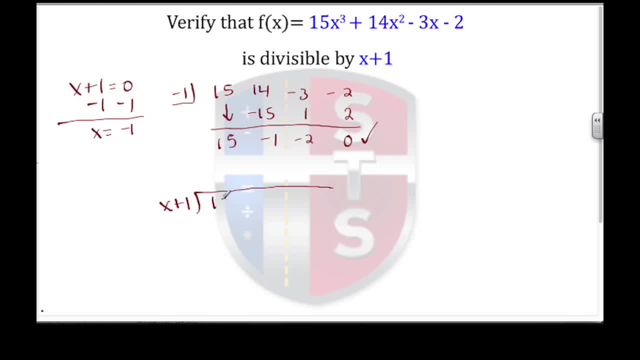 And then we list the function f of x, So 15x cubed plus 14x squared minus 3x minus 2.. We begin by trying to eliminate this x cubed term And we see that we'd have to multiply x by 15x squared. 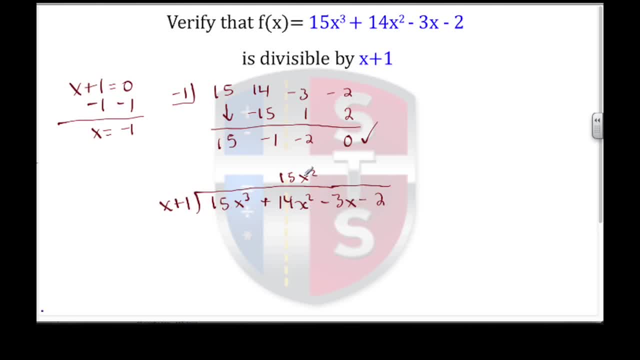 And that would give us a 15x cubed. So now, 15x squared times x would give me 15x cubed. Times the positive 1 to give me a positive 15x. Then I end up doing subtraction. I know that each one of the signs for these terms have to change. 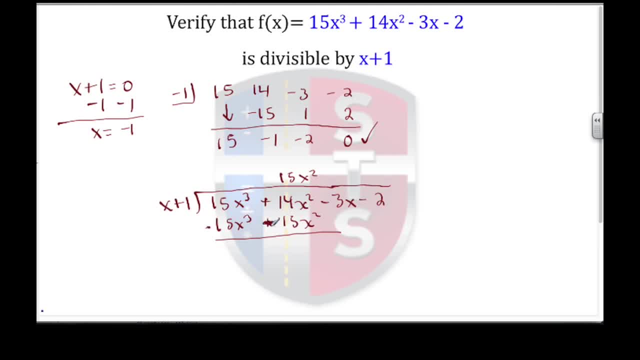 So that's a negative. And this positive here also becomes a negative When I subtract these first two terms go away, which is what I want to happen. Now I have 14x squared minus 15x squared, to give me a negative x squared. 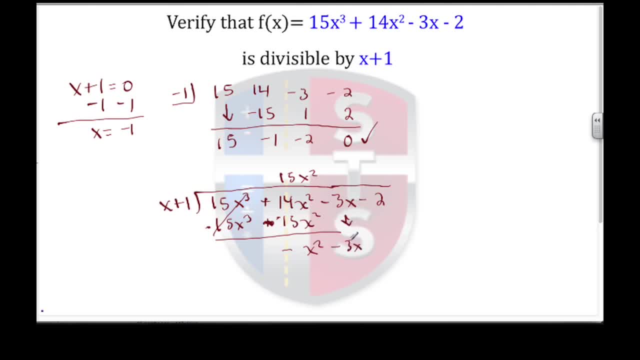 Then I bring down my negative 3x and I continue by asking myself the same question: What do I need to multiply x by to end up with a negative x squared, And in this case that would be a negative x. So now negative x times negative x will give me a negative x squared. 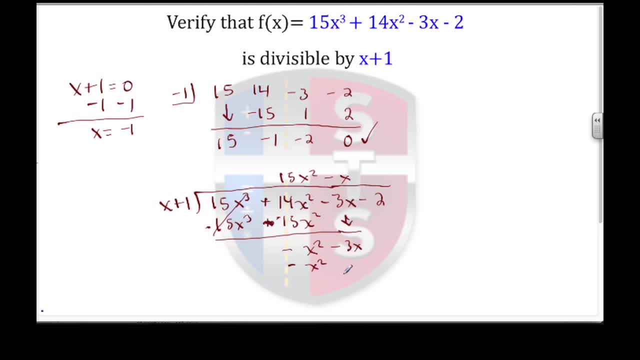 Negative x times a positive 1 will give me a negative x And I have to distribute a negative to both of these terms, So they're negative and that means they become positive Again. my first two terms here cancel each other out and I'm left with negative 3x plus x, which gives me a negative 2x. 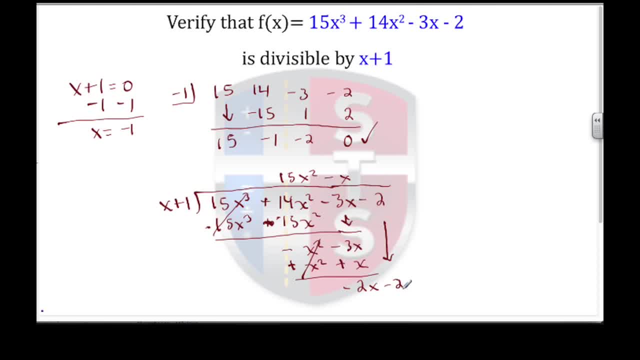 And then I bring down my next term, which is a negative 2.. And finally, I ask myself the same question again: What times x will give me a negative 2x? And in this case that would be a negative 2.. 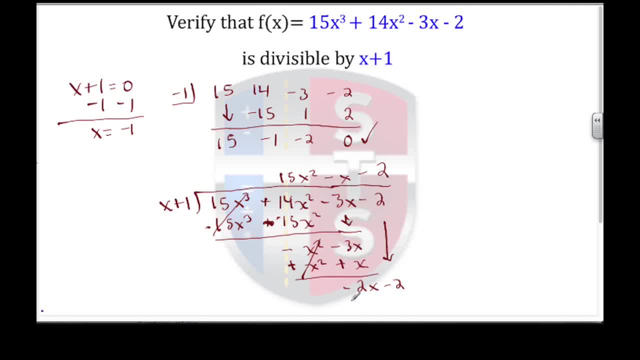 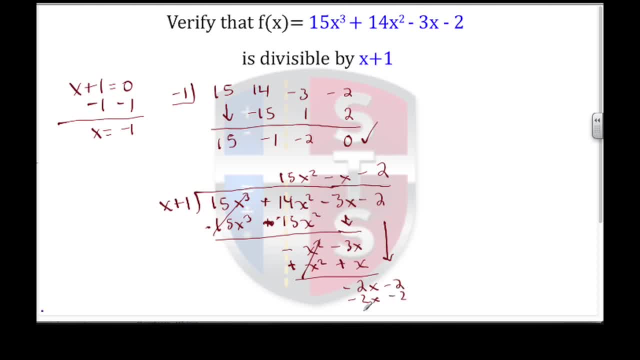 Negative 2 times positive. 1 gives me a negative 2.. Again, when I subtract, the terms change their sign, because I distribute a negative And we see that I come up with a remainder of 0, which matches my answer up here. 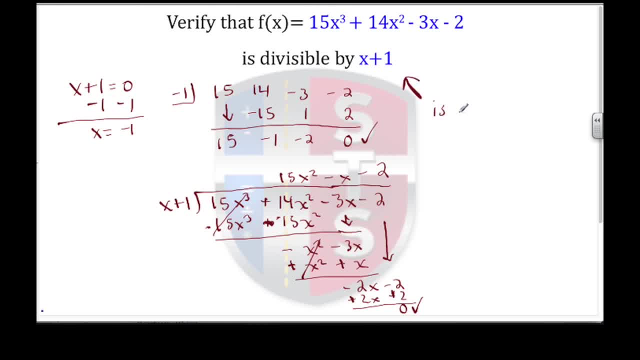 So I know that x plus 1 is a factor. So that sums it up for this video from Speller Tutorial Server. If you want to learn more about Speller Services, please friend us on Facebook and also subscribe to our YouTube channel, both found under the name Speller Tutorial.